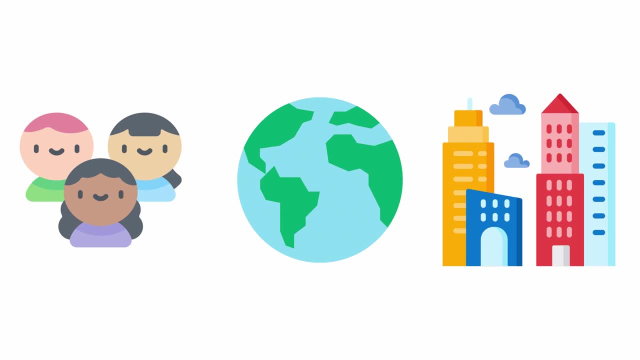 needs, not just today, but in the future as well. This means we must use Earth's resources in a way that can be used forever. If we use too much of something today, it could be gone forever. To do this, there are three main areas. 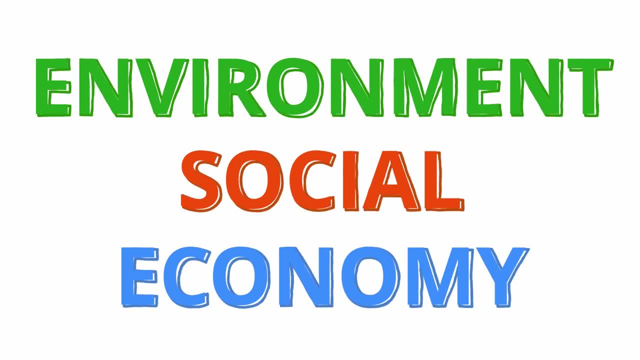 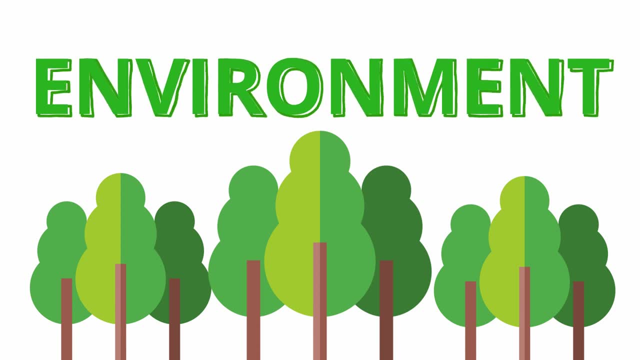 There are three areas known as pillars to focus on: Environment, social and economic. When we talk about environmental sustainability, we mean using Earth's resources in a way that they have enough time for Earth to replenish as we use them. This can mean something like trees. 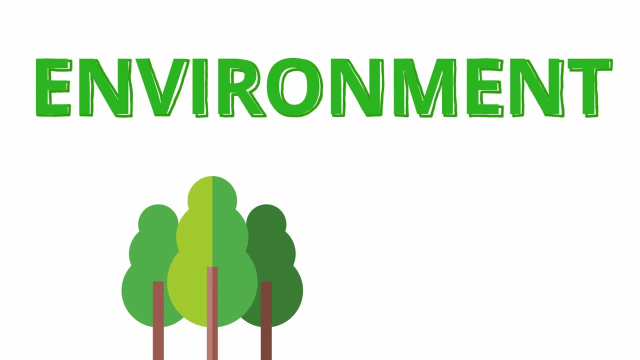 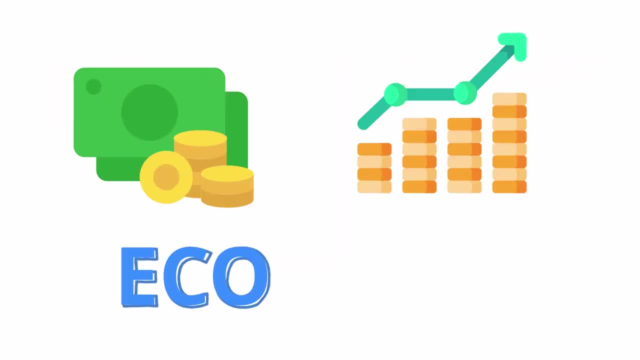 where we cut down too many and don't plant enough to replace them, or by creating waste streams faster than Earth can absorb them, causing waste to build up. Economic sustainability is where people are able to make enough money to support their needs and businesses. It's about the continued success of the economy for all people. 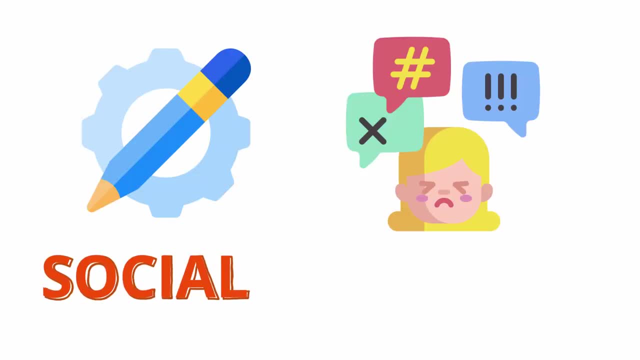 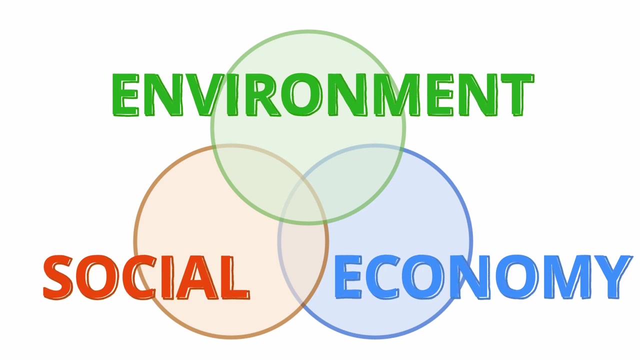 And social sustainability is where all people have the opportunity to get the resources and economic success they need while not facing any exploitation or discrimination of any kind. These three pillars may sound pretty similar to you, and they should, because they overlap and impact each other. For example, businesses want to make more money, but often have negative 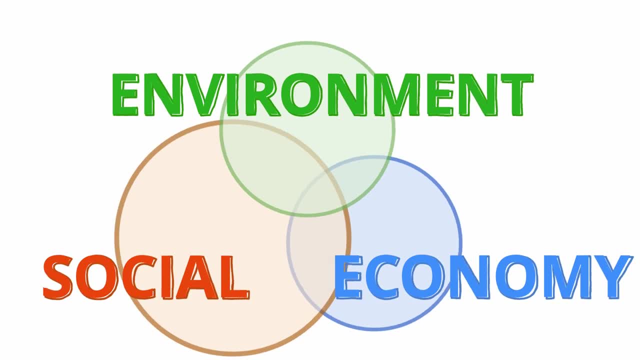 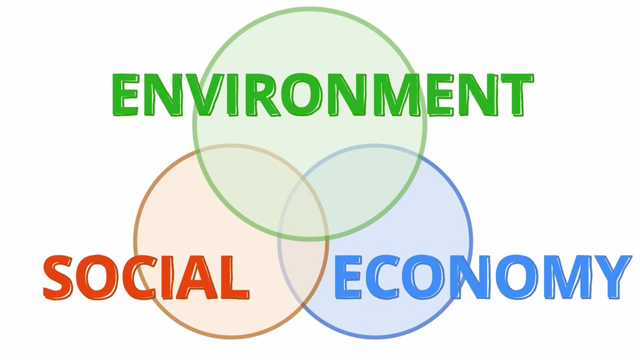 environmental and social impacts in doing so. Socially, people want to support their families, but that often means limiting business and environmental impact. And environmentally, we need to use Earth's resources sustainably, but certain groups of people and businesses don't want to limit their consumption. 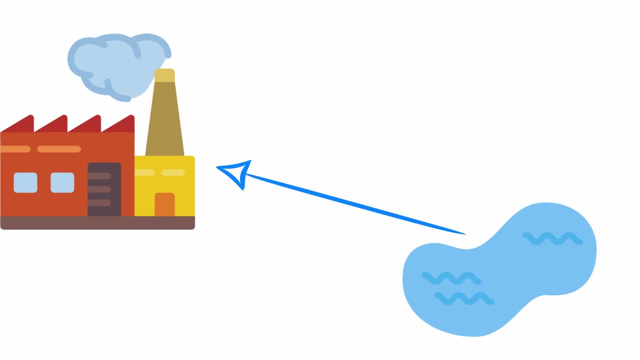 To make this easier to understand, imagine a business that uses a lot of Earth's resources, for example water from a nearby lake. If that business uses water from the lake too quickly, it's possible to use up all of the water and the lake will be gone, which means the people who live. 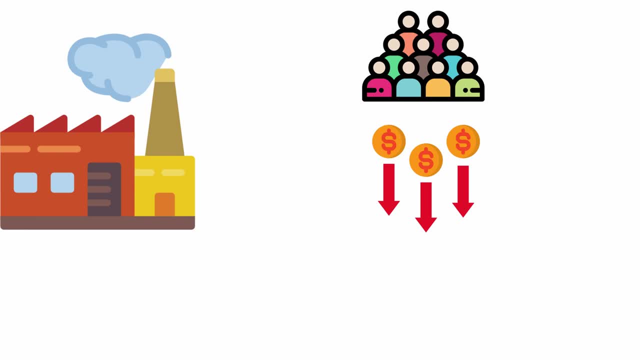 will have access to water and will have to find it elsewhere. Also, without any water, the company won't have the resources it needs to make its products. This decision by the business may have been beneficial in the short term, but in the long term it didn't last and resulted in 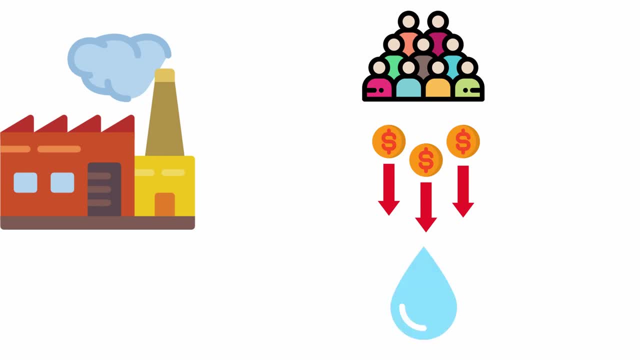 negative impacts on people, profit and planet. This could have been prevented, but the business put profits first and the needs of people and the environment last. However, if the business found ways to use less water and therefore reduced its water consumption to an amount where the lake